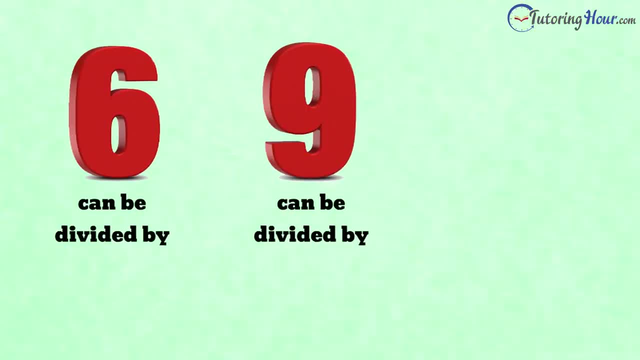 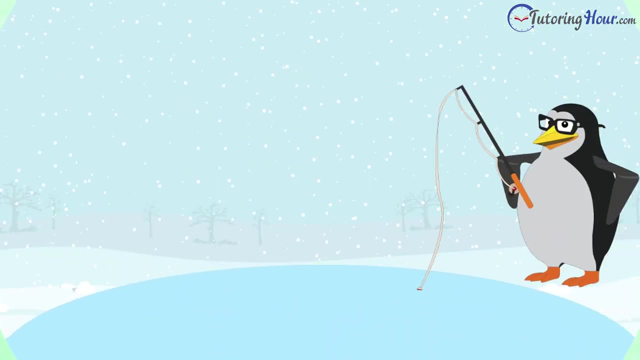 The numbers six and nine could be divided by other whole numbers, But seven could only be divided by one or itself. From this we understand that six and nine are composite numbers and seven is a prime number. Let's take a look at the first few prime and. 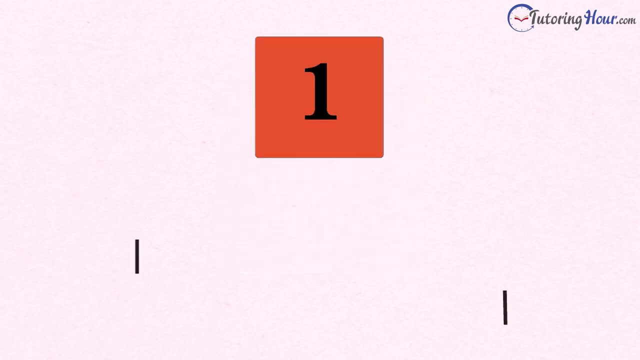 composite numbers. Take the number one, for instance. It is neither prime nor composite. Let's move to our next number two. It has only two factors, which are one and two. There are three factors in the number two, just like the number of five. 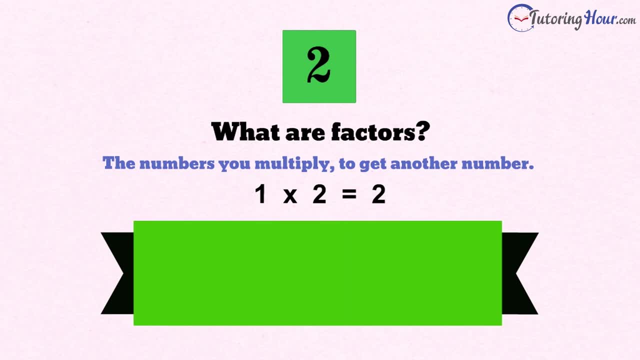 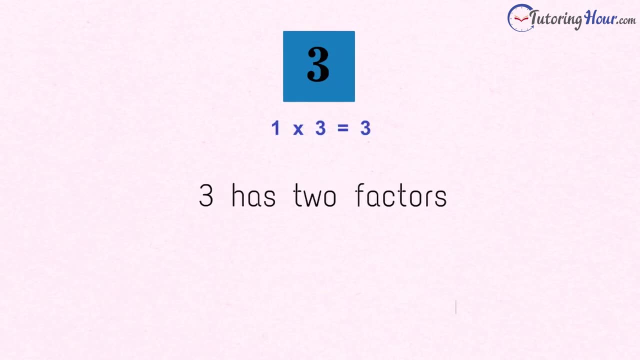 They are nothing but the numbers you multiply to get another number. We multiply one and two to get the number two. So one and two are the factors of two. Now let's check the number three. Three has two factors and they are one and three. Our next number is four, which has three factors. 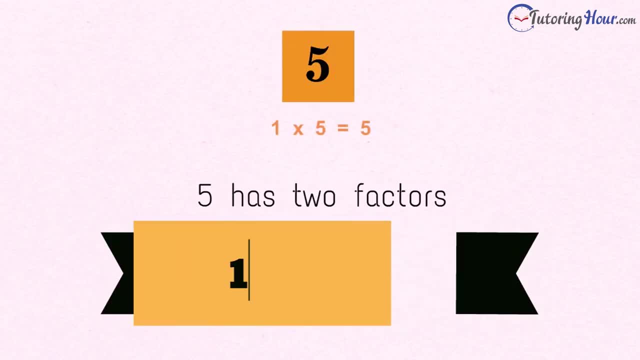 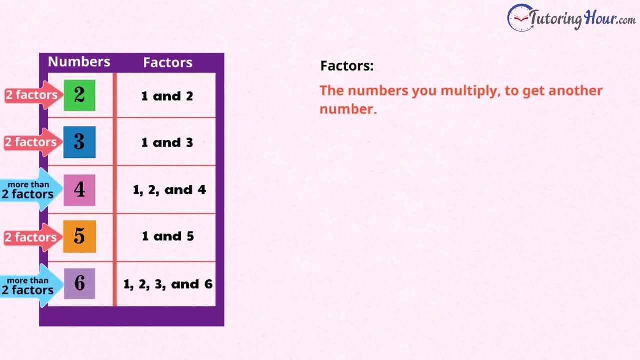 one, two and four. While the number five has just two factors, Then the number 6 has 4 factors: 1,, 2,, 3 and 6.. Look at the numbers here. some have 2 factors and some have more than 2.. 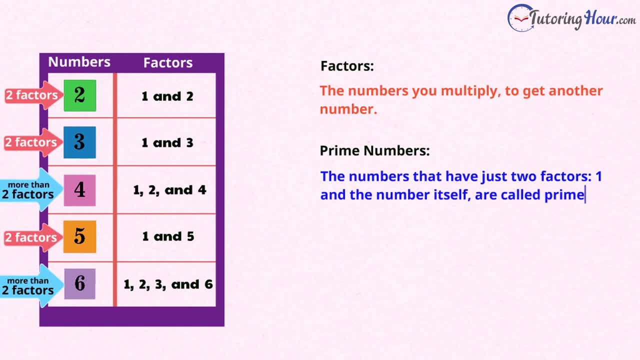 The numbers that have just 2 factors- 1 and the number itself- are called prime numbers. The numbers that have more than 2 factors are called composite numbers. But with larger numbers the quickest way to find the factors is by using the divisibility. 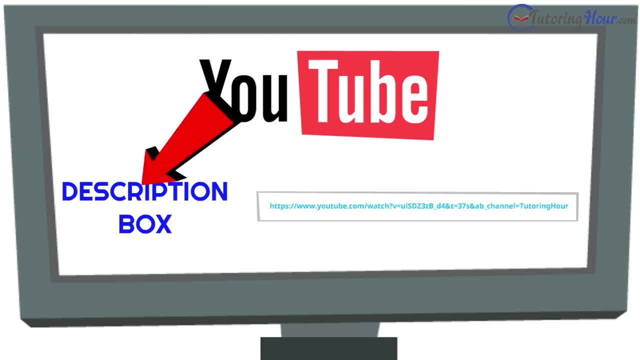 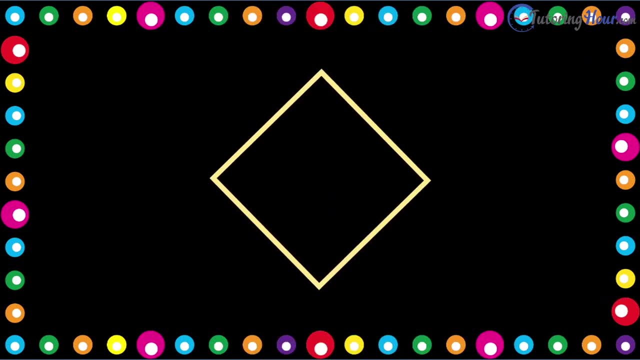 rule. If you are not sure what they are, go ahead and find the link to our video on divisibility rules in the description box. Moving on, let's show you an interesting way of finding prime numbers using the sieve of Eratosthenes. 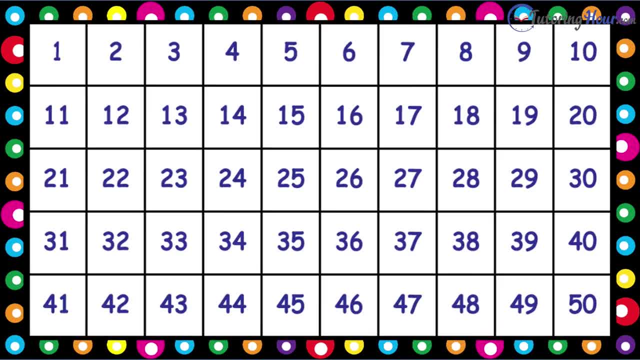 We'll use this chart with numbers 1 to 50.. Let's cross out 1 and green. We know it is neither prime nor composite. 2,, we know, is a prime number. In fact, it is the only prime number. 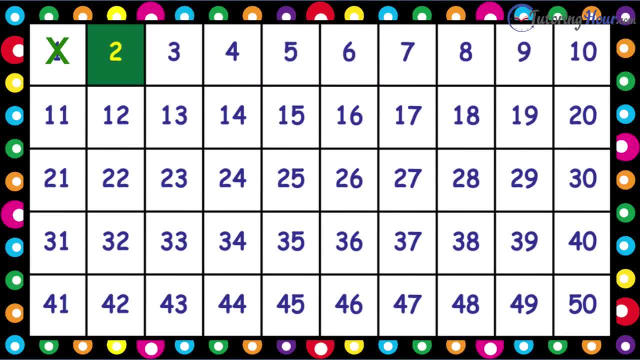 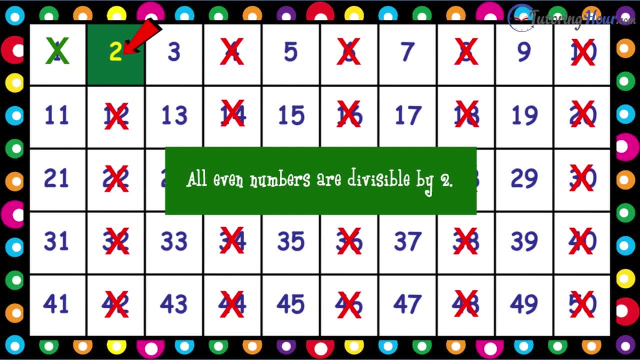 2, we know, is a prime number. In fact, it is the only prime number. 2, we know, is a prime number. Now let's cross out all the multiples of 2.. In other words, all even numbers, since they are divisible by 2.. 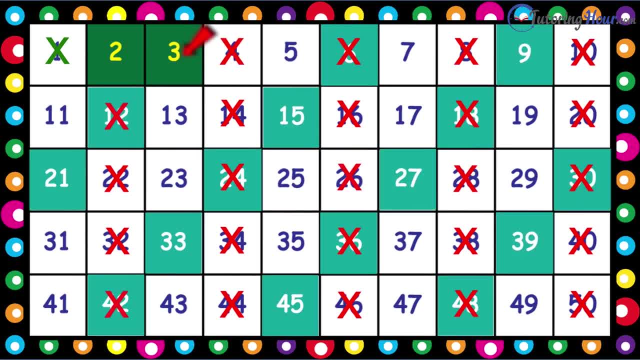 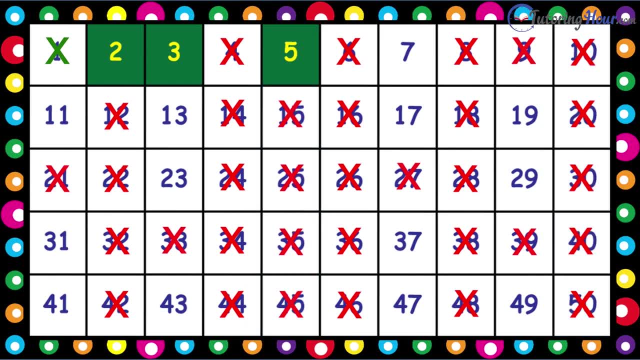 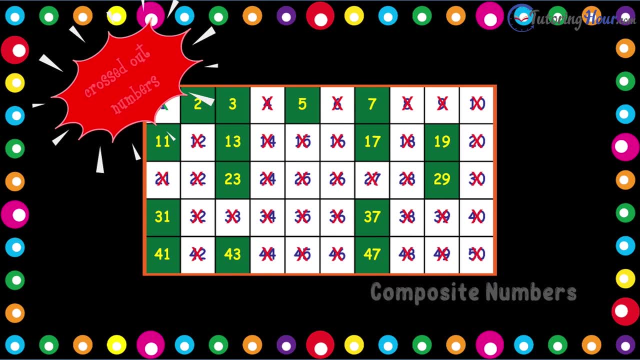 3 is our next prime number. We'll cross out all its multiples. 5 is a prime. We need to cross out all its multiples as well. We'll highlight 7 and eliminate its multiples. All the numbers that are crossed out in red are composite and the numbers left are the. 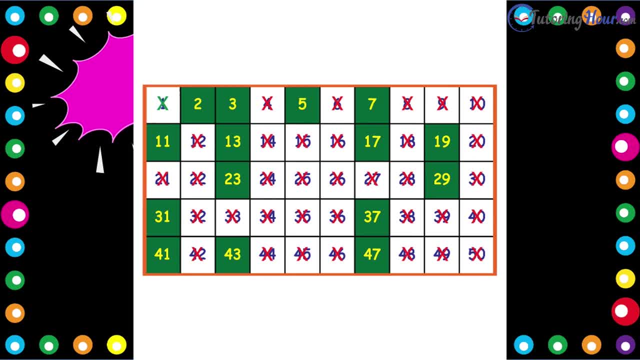 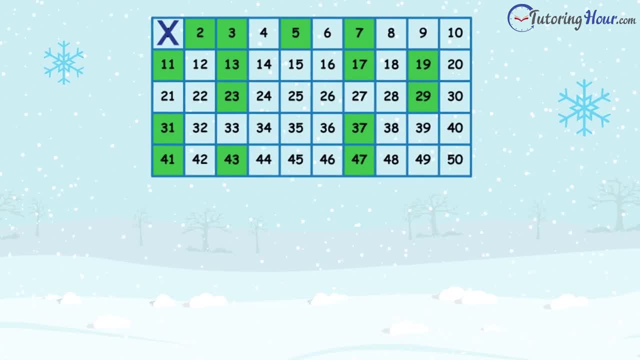 uncrossed, or obviously, prime. We have clued you enough on how to find the prime and composite numbers between 1 and 50. Go ahead and extend this method to any number and scout out the prime and composite numbers in no time. 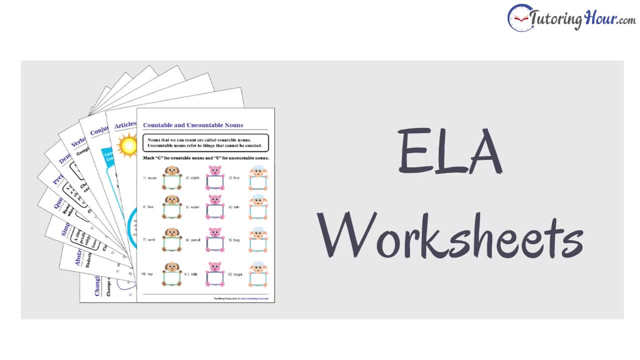 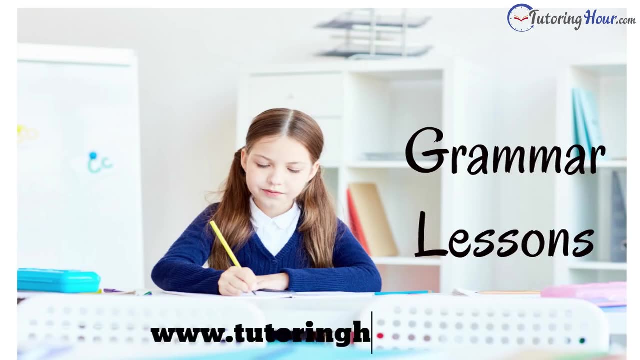 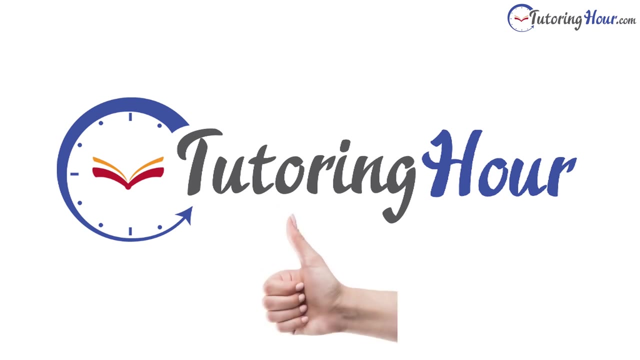 There is nothing like good practice to fill the gap between learning and doing. If you guys got some time on hand and think you must practice this stuff, then visit our website TutoringHourcom. Check the link in the description box, download the worksheets and get started. 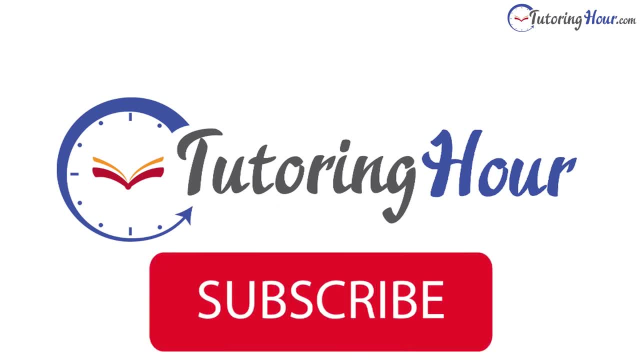 Don't forget to like our channel and hit the subscribe button if you haven't already done that. Thank you guys for watching Tutoring Hour. 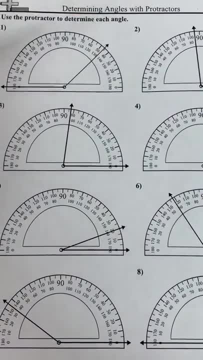 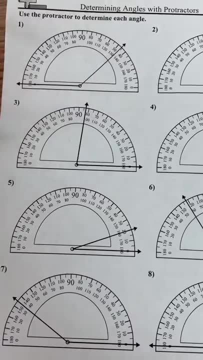 Hi guys, it's Mrs Fortuna. I'm here to teach you today how to read the measurement on a protractor. A protractor is a tool that we use to measure angles On the EOG or on any assessment. you won't. 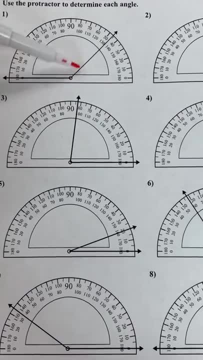 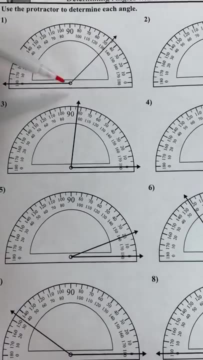 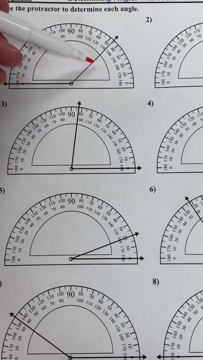 actually be handed a protractor. You'll see it pictured like this, with the angle already put on the protractor. And here's what you need to do. Step one is you look at the angle and you say: is it acute, obtuse or right? Well, this angle opens up really large. So I know this is an obtuse. 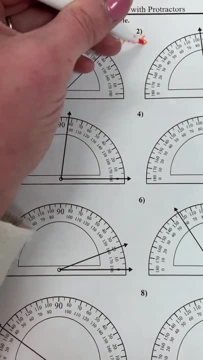 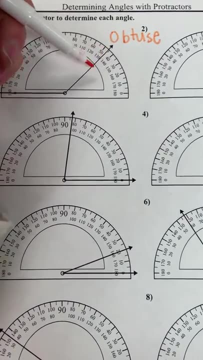 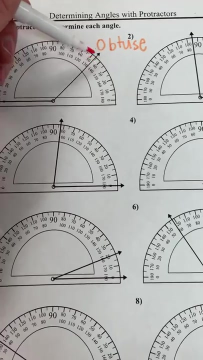 angle. so I label my angles. This helps me determine the measurement. Then I take a look and see: well, where is the angle reading? You can kind of see there's two measurements here. One is between 40 and 50. Anywhere within five is okay. So for this sake we'll say: